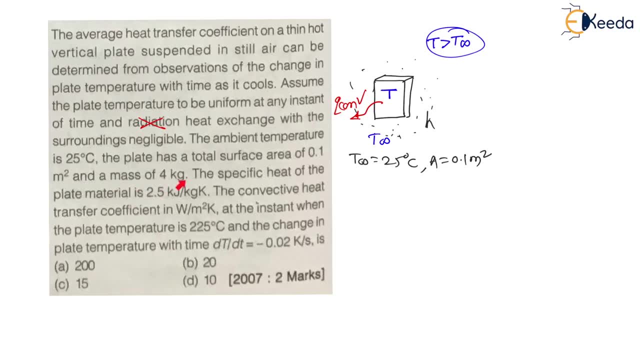 square. then then, and the mass is 4 kg. the mass of this plate is 4 kg, therefore M is equal to 4 kg. then the specific heat of the plate material is 2.5 kilo joule per kg Kelvin. therefore here specific heat, CP is given 2.5 kilo joule. 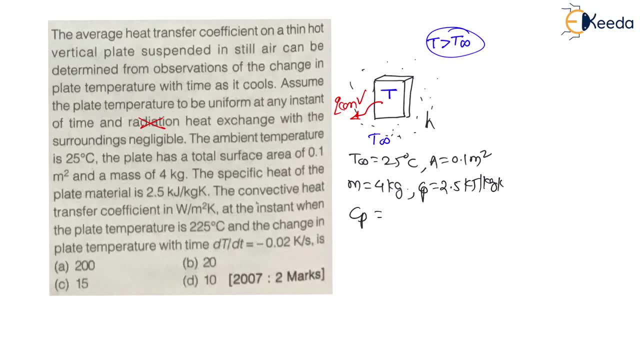 per kg Kelvin. therefore, can I write: CP is equal to in kilo in joule per kg Kelvin. let us convert: it will become two, five, double zero, two thousand five hundred joules per kg Kelvin. right then, the convective heat transfer coefficient in watt per meter square Kelvin, the C H convey to transfer quotient dh in watt. 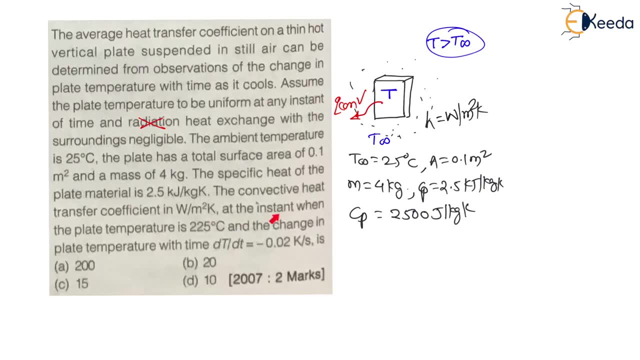 per meter square Kelvin. add the instant when plate temperature is 225 degrees Celsius, when display temperature is 30, is equal to 225 uses. yes, in this convective transfer coefficient we have to find, and the change in plate temperature with time, that is, dt by dt, is minus 0.02 kelvin. 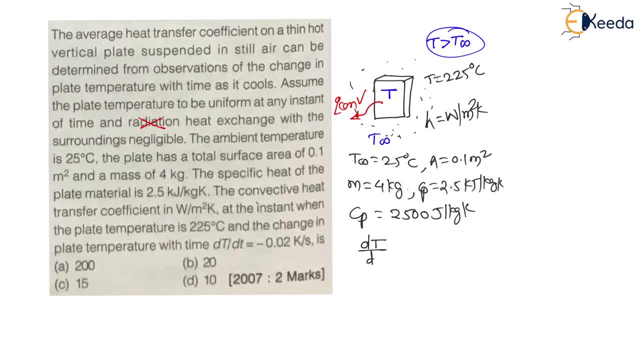 per second. now here, dt by dt, change in plate temperature with respect to time is given minus 0.02 kelvin per second. now, my dear students, let us understand the simple way now why this is minus. it is minus because, with respect to time, the plate temperature is decreasing. 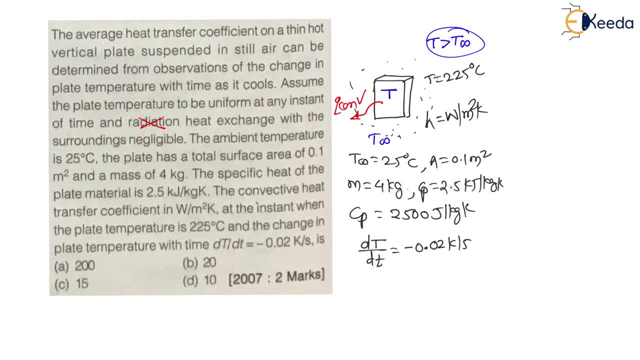 means, as the time is increasing, the plate temperature will decrease. because of this, this dt by dt is minus right now. my dear students here, let us understand the mechanism of heat transfer, how the heat transfer will be there now, as this plate temperature is more than surrounding fluid temperature, then, with respect to time, slowly, slowly, this plate temperature will decrease. 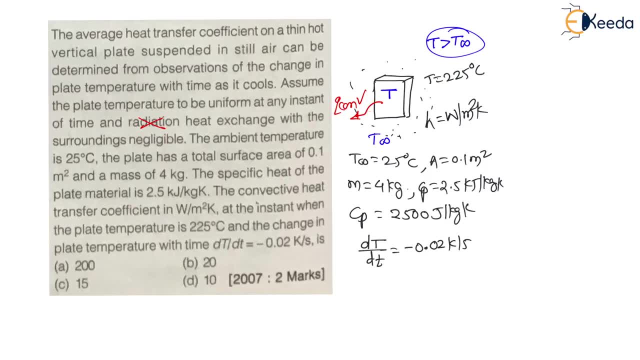 the plate temperature is slowly, slowly decreasing. right means whatever may be. the heat loss from this plate is going into the surrounding plate temperature is going into the surrounding by convection and can i say, the heat loss from the plate is equal to change in energy of this. 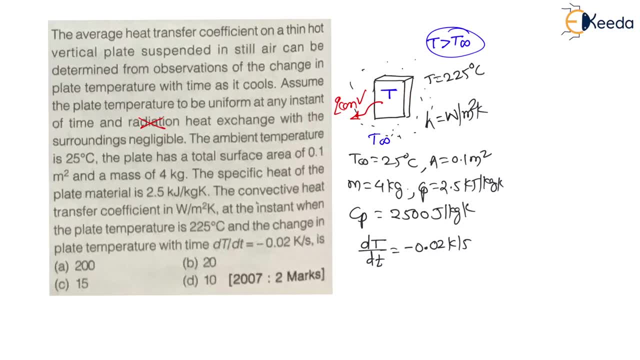 plate. that is decreasing energy of this plate. therefore, my dear students, the simple equation we can say: the heat lost, it lost from the plate by convection, by convection is equal to decrease. in is equal to decrease in internal energy, internal energy of plate plate. right, definitely, as temperature of plate is slowly, slowly decreasing the internal energy. 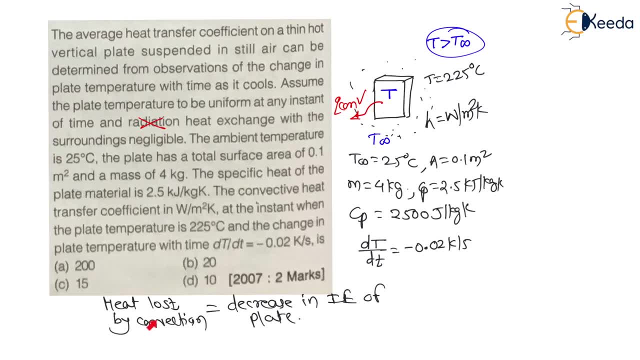 of plate will decrease. therefore, the steady flow energy equation or steady state equation, we can say: whatever may be the heat loss must be equal to decrease in energy of this plate, right? so let us equate them and let us find the answer now, my dear students, note down: 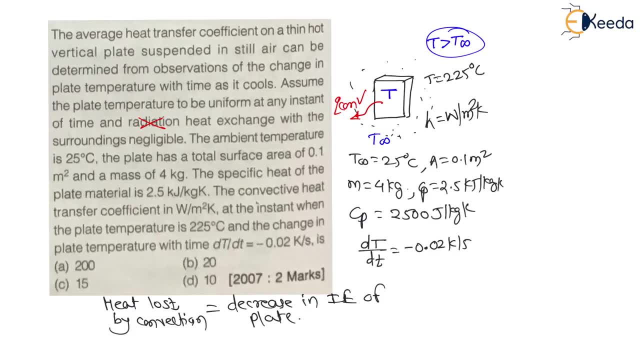 these options right, because i am going to erase this question. i will tell you answer. answer is option d, that is 10, right now. let us pause this video. pause this video and check whether you are getting this 10 or not. now let us delete this question right, so that? 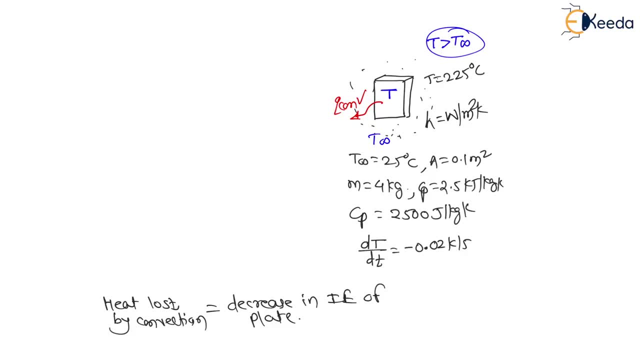 we will get sufficient space for the solution. now, my dear students, let us check what is happening here now. heat lost is nothing but heat loss by convection, which is nothing but h, a delta t right is equal to now. this answer is wet. this answer is wet. now it could change. 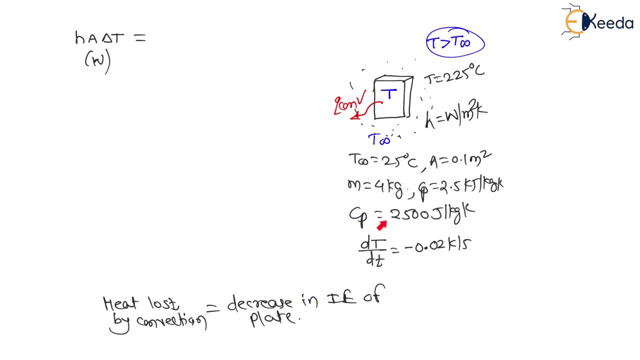 in internal energy. now, my dear students, change in internal energy will be emcp, d by dt, emcp, dt. let us say emcp divided by d, t c, pd by d, t, c, pd, d by d t. let us say e m c, p, d t, c, p d. 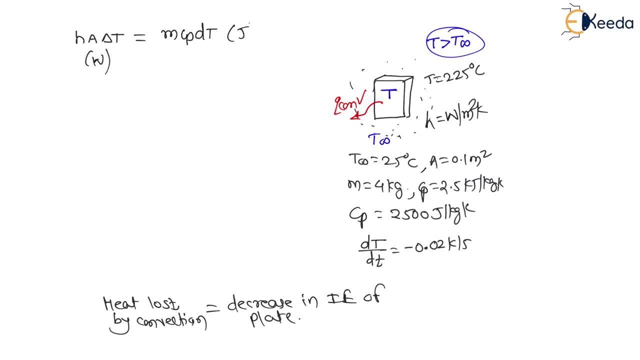 d, t, c, p, d t. now, if i can take any energy in my internal energy, it is equal to d. the energy dt is nothing but joule. it is joule and if i divide with time that is dt, it will become joule per second, which is vat. right? this is change in internal energy, right? so, my dear students here, 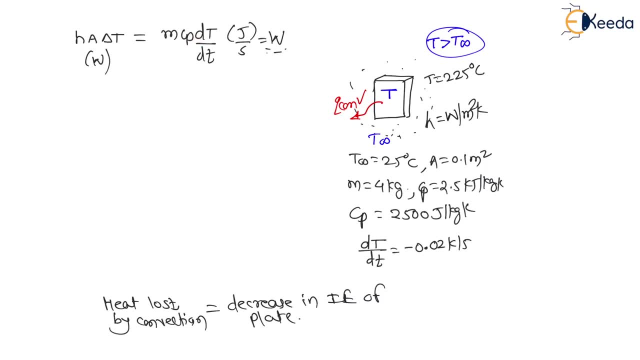 this is a heat loss and this is a change in internal energy. right, therefore, can i say: heat loss from the system is negative. therefore, it is whenever heat is losing from the system. it is negative. therefore, i have to write here negative sign or you have to consider this positive and